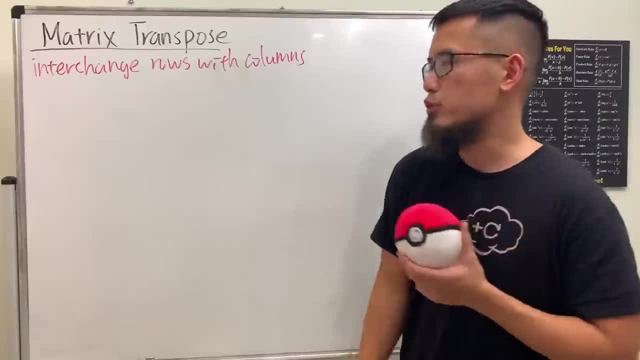 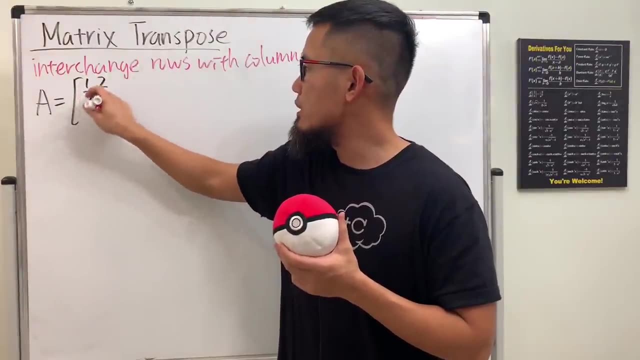 And let me give you guys an example real quick, and this right here works for any size matrix. So let me say A is equal to a 2x4 matrix. let's say we have 1,, 2,, 3,, 4,, 5,, 6,, 7,, 9.. 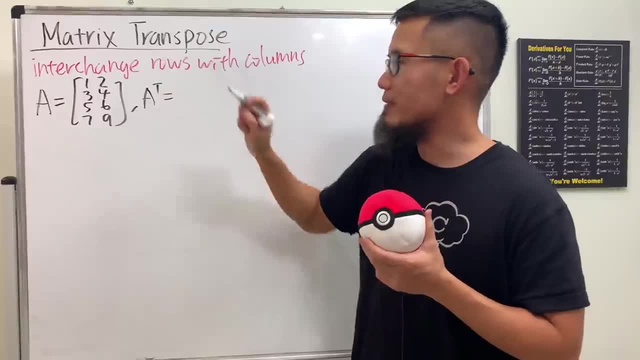 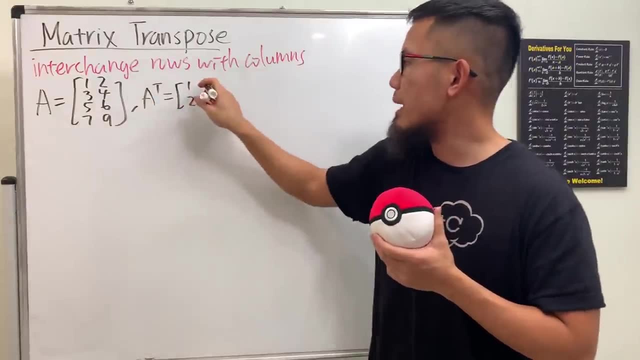 In that case, our A transpose is going to be the following: We take this row and put it as a column, so we have 1, 2, and then this will become 3, 4, and then 5, 6, and then 7, 9,, just like that, right. 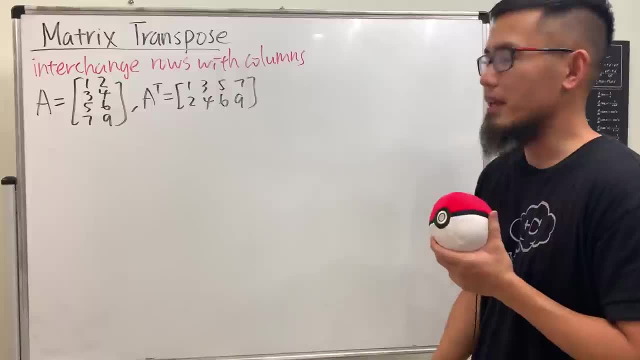 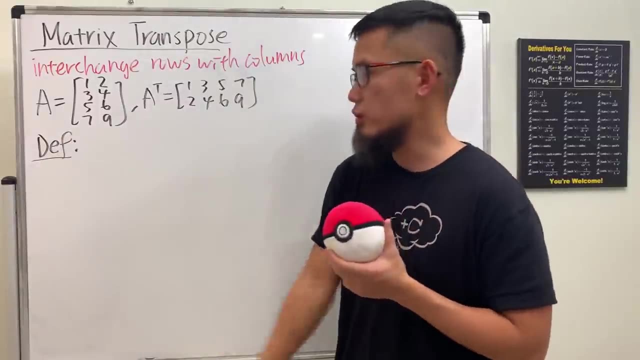 And if you have a square matrix, it's pretty much the same thing, And here's the key notation that you have to know, right? So this is the definition in terms of using the notation for that. Well, pay attention to the entries. 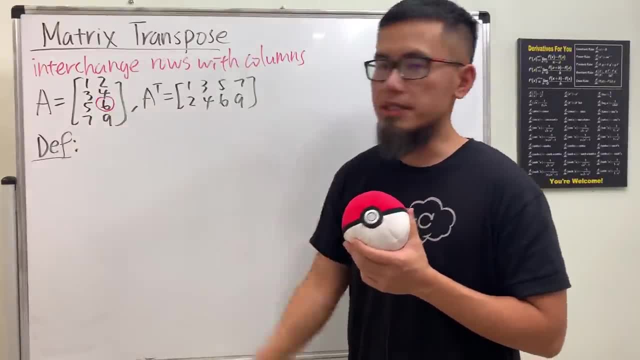 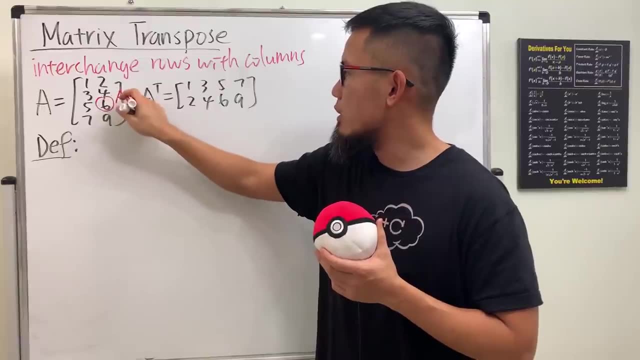 For example, if you look at the 6,, where is the 6?? This is in the 3rd row, 2nd column, so we will write this as A 3,, 2, right. And now, where is the 6? right here. 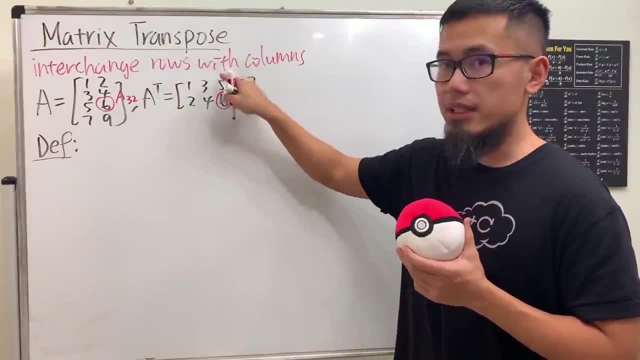 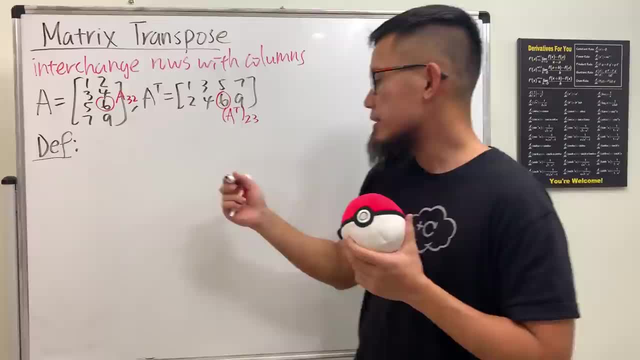 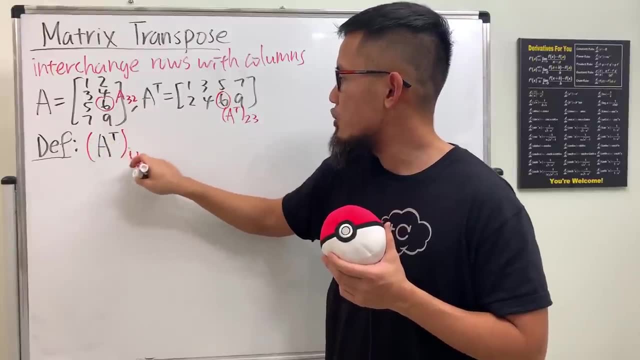 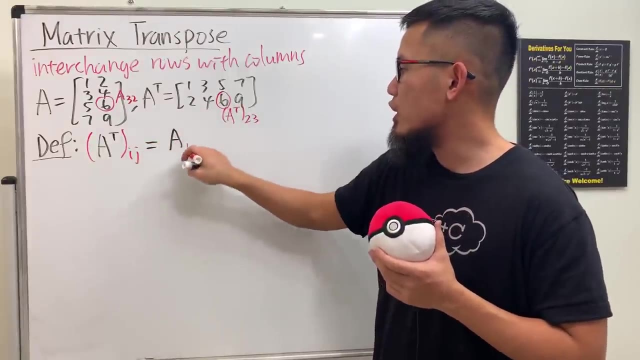 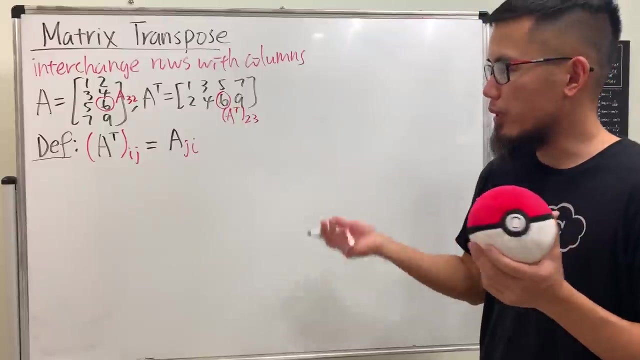 row, third column: all right, so here's the deal. if you have a, transpose this right here. if you look here, it's i- j's entry. this is actually the same as look at the a matrix, but you look at the j- i entry. so this right here is the key. and there are some properties and i'm going to write down a few. 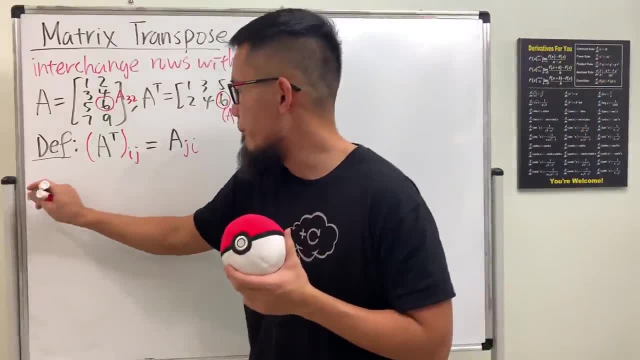 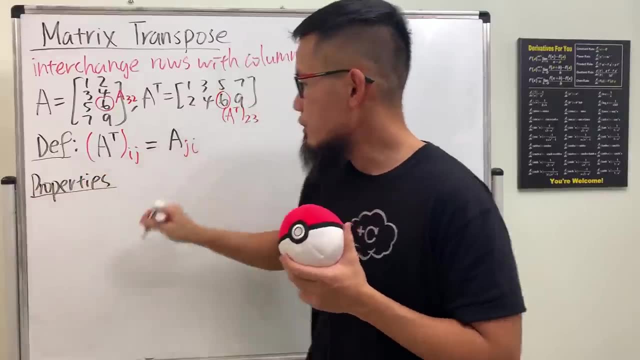 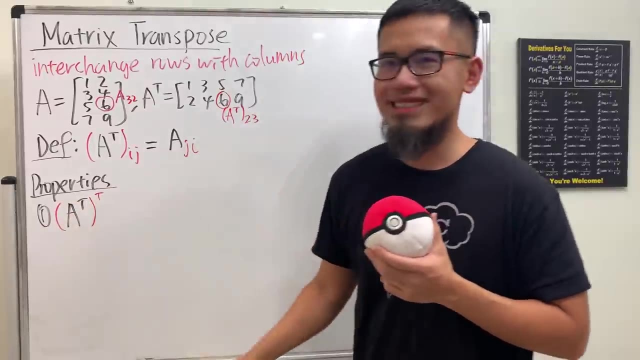 of them, and i'm going to prove one for you guys. so here we go. here are some properties that you should definitely know. properties first one: imagine if you have a transpose already, but you do the transpose again, and what will happen? we do the transpose. if we do it again, then pretty. 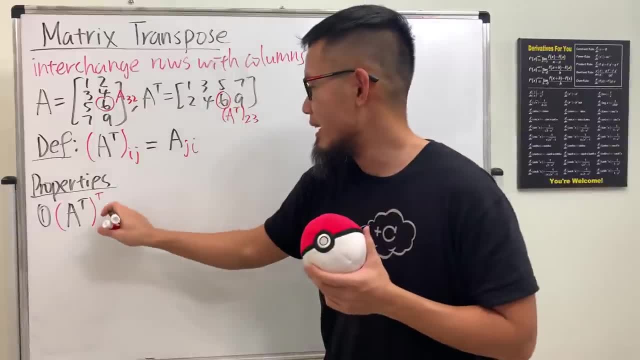 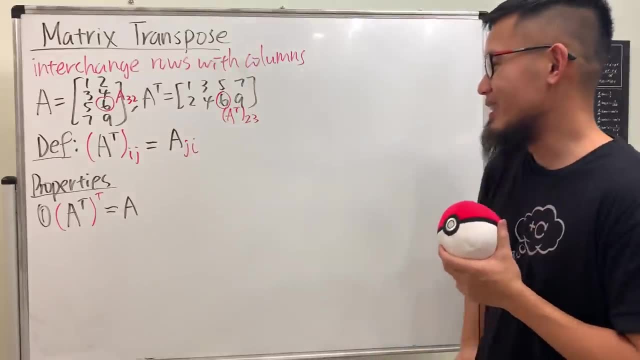 much. we'll just go back to the original, right. so that's pretty much it, and i think it's pretty clear. so i'm not going to prove that and, in fact, in my opinion, uh, the proofs for the super obvious statements are actually pretty hard, so let me not prove that. 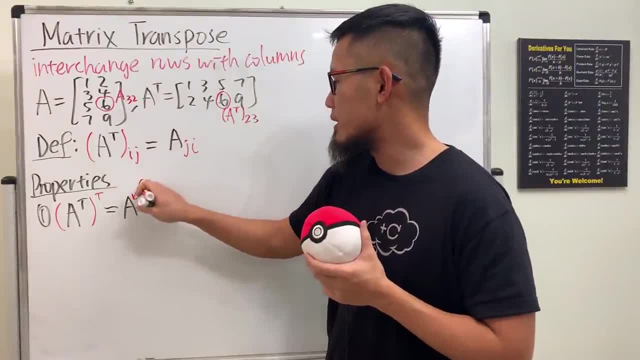 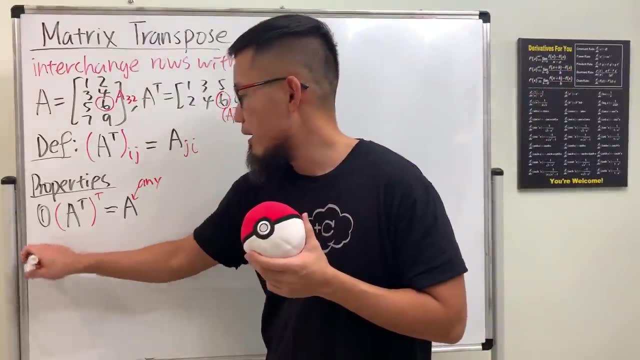 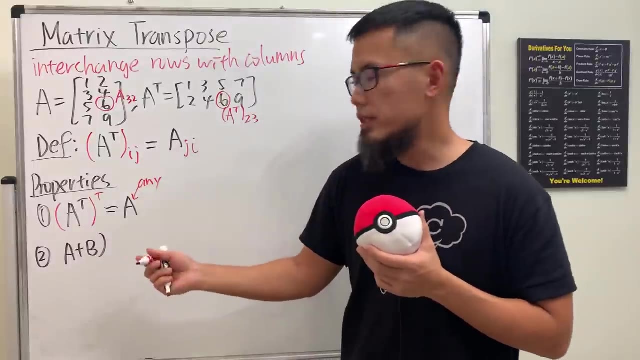 but anyway, though this right here works for any matrix, right, it works for any matrix. it doesn't have to be square matrix, all right. second, one suppose let's look at two matrix adding up together, right, so the sum of two matrix, and of course when we are adding we have to make sure that they have. 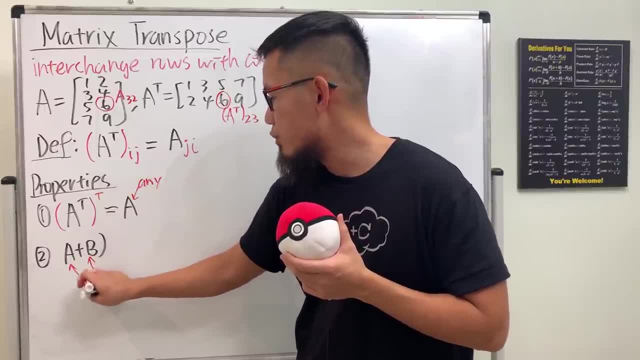 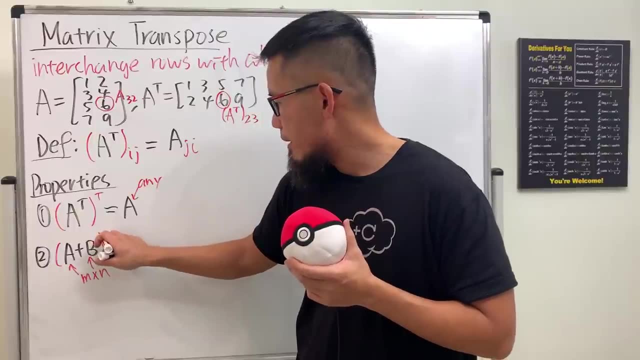 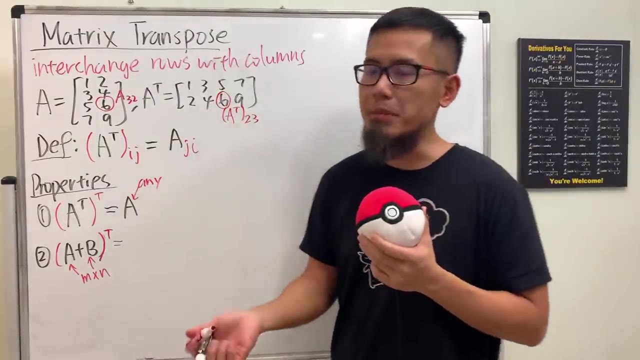 to have the same dimension. so let's say both of them have to be, you know, m by n. of course it can be square as well. anyway, after we add them, let's then do the transpose. in that case, if we add first to the transpose, it's actually the same as we do the transpose and then add, so we have a transpose. 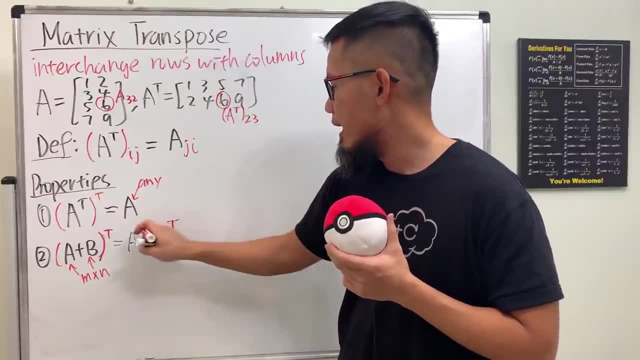 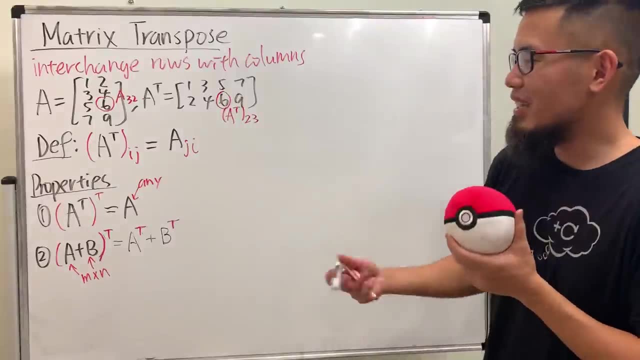 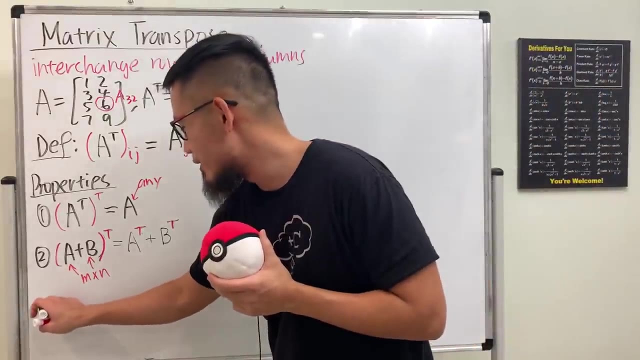 plus b transpose, and i think this right here is fairly obvious as well. so i'm not going to prove this one either. you can just test out some examples, then you'll see. oh, it works really nicely. yeah, so that's that idea, all right. third one- and you guys may be wondering: which one am i going to prove, right? 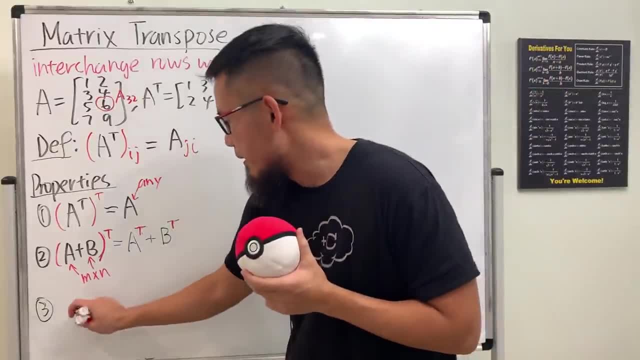 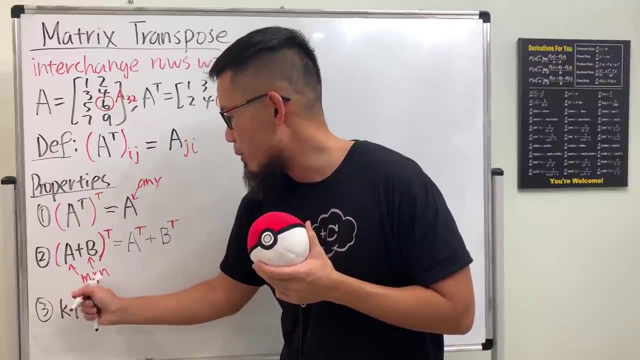 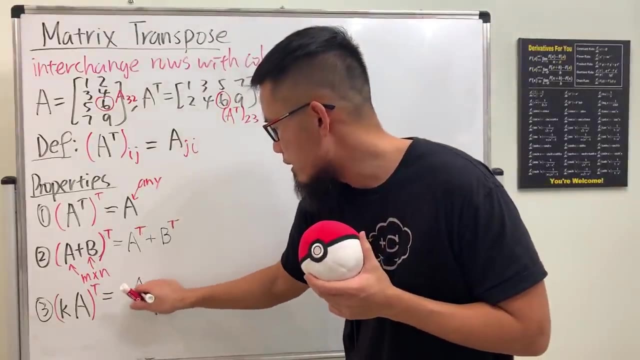 i am going to prove one for you guys. for sure, all right, if you have a and before you do a transpose, you multiply by some constant, let's say k, and then you do the transpose. all right. well, this right here, it's actually the same as do the transport first. so a t, right here. 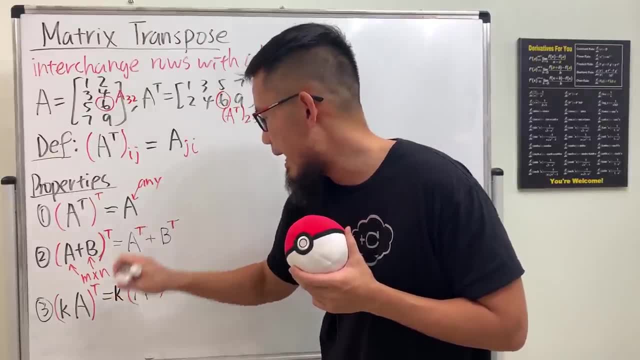 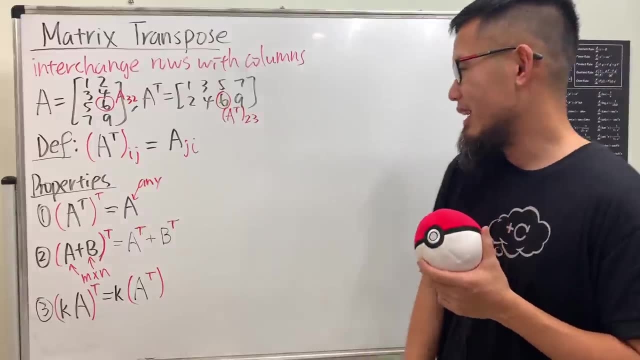 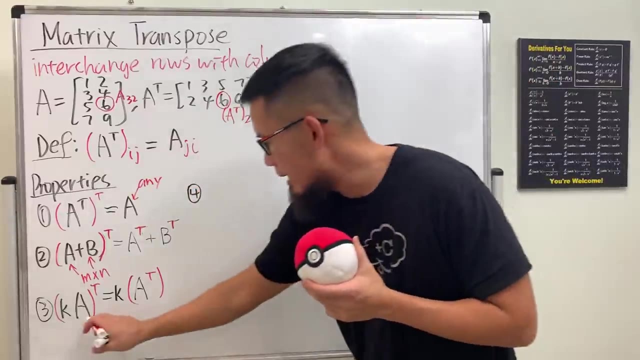 and then multiply the result by k. that's, uh, actually also legitimate. it's also pretty obvious, in my opinion, but just keep that in mind as well. now we have a couple more slightly more interesting ones. number four: let's talk about product. by the way, this right here works for any matrix, right. 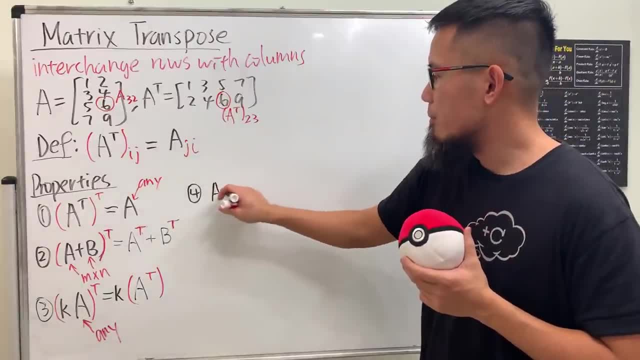 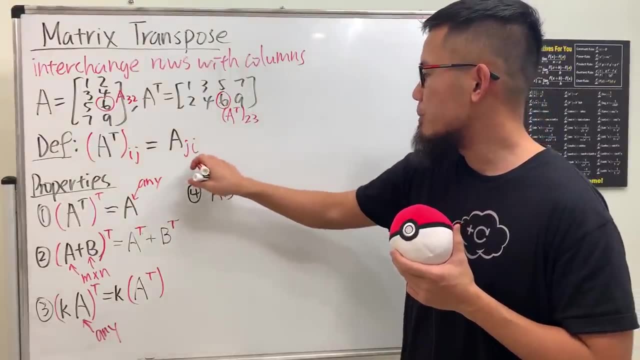 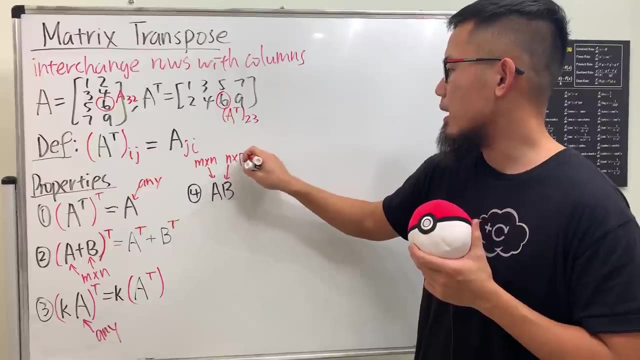 number four. let's look at product a, b. in this case we have to make sure that, well, the dimension of a has to be, let's say, m by n, and let's say dimension of b has to be starting with n and multiply by whatever right and by p, for example. anyway, just make sure the 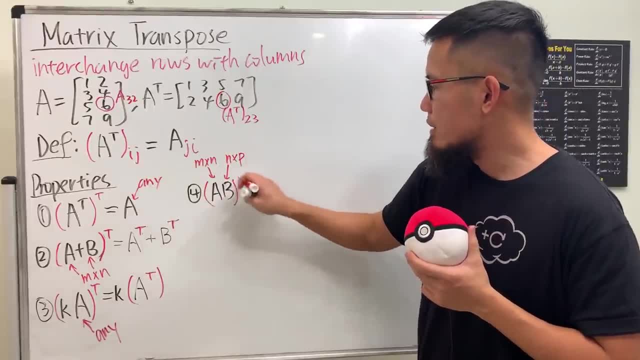 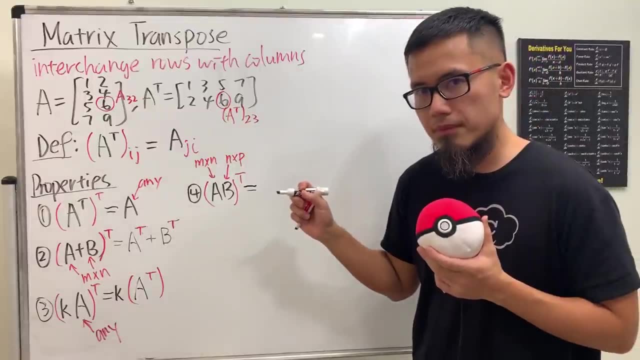 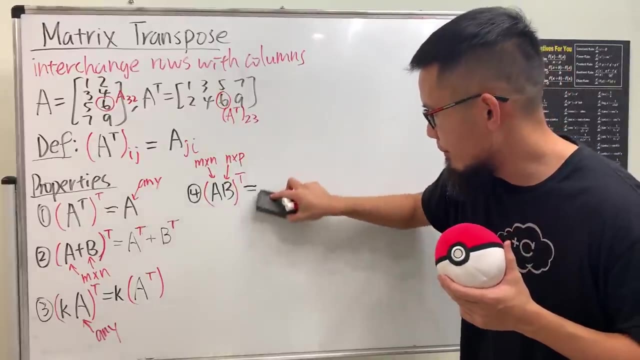 dimension works. and then if you have this and do the transpose, if you think that a, b transpose is equal to a transpose, b transpose, then let me tell you it's wrong. and this right here might be kind of weird, yeah, because when you multiply matrices, it's weird, right? this right here is: 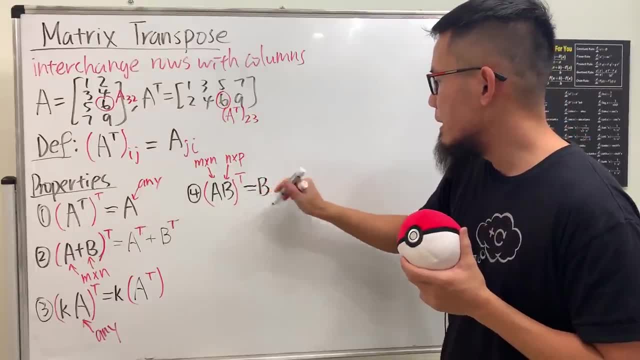 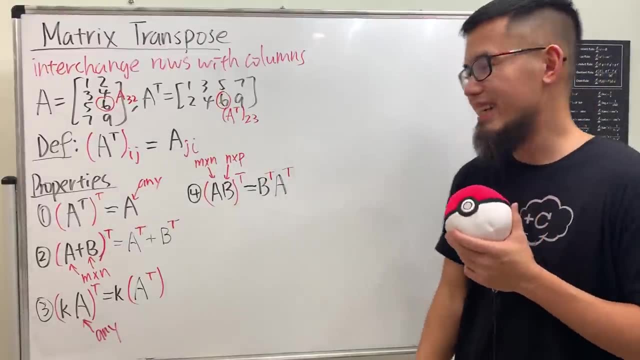 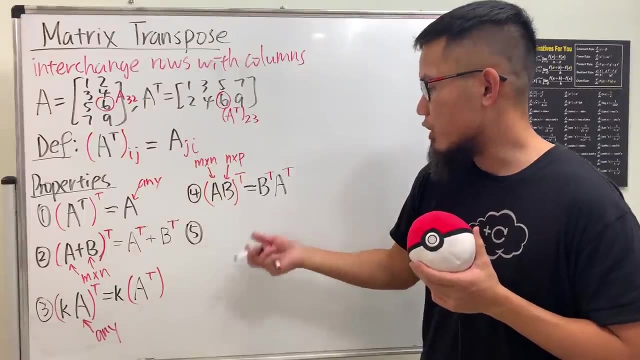 actually the same as b transpose times a transpose, and this is the one that i will prove for you guys. right, and then number five. another thing i can notice is that this one, of course, have some, is that, well, if you can find the determinant of a matrix where the matrix is, uh, square, so if you 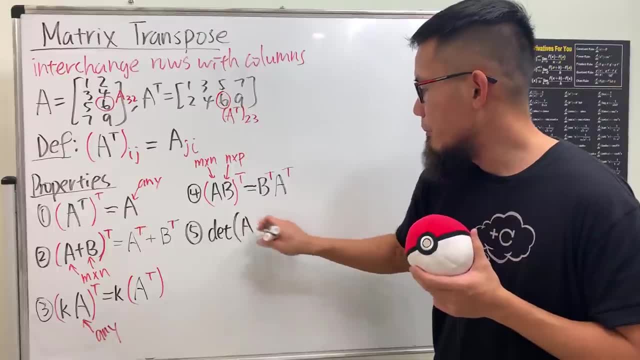 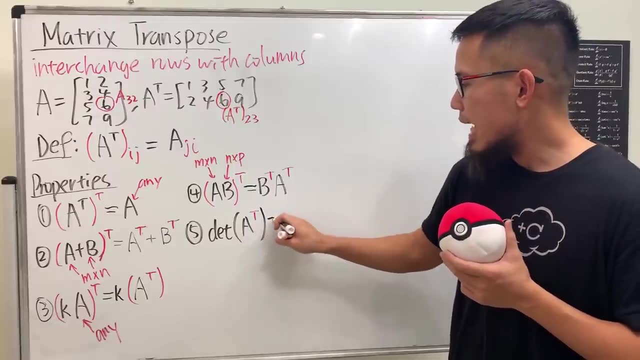 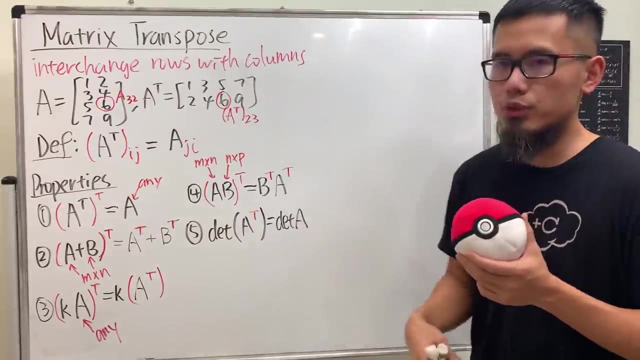 have the determinant of a matrix. but let's say you look at its uh transpose first. right, the determinant of the a transpose, it's actually the same as the determinant of a right. uh, i think this one is also fairly okay to prove. you can just use the cofactor, expansion, the determinant, etc. right? 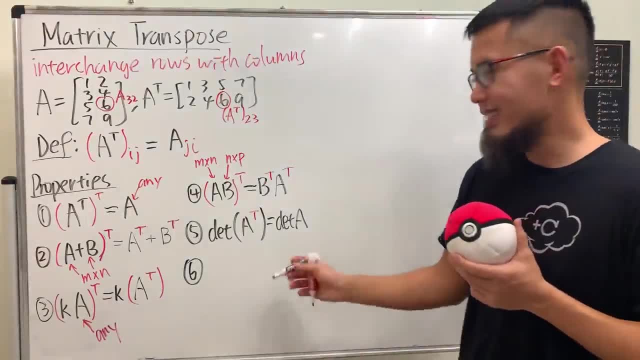 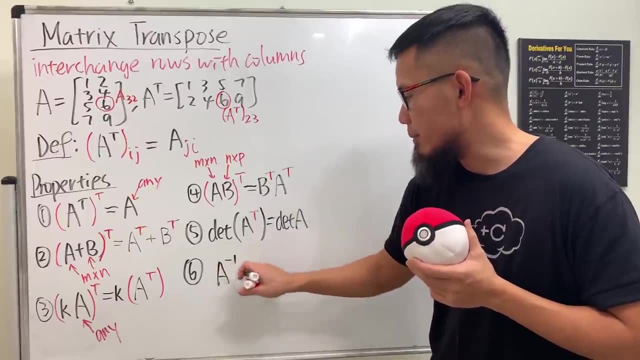 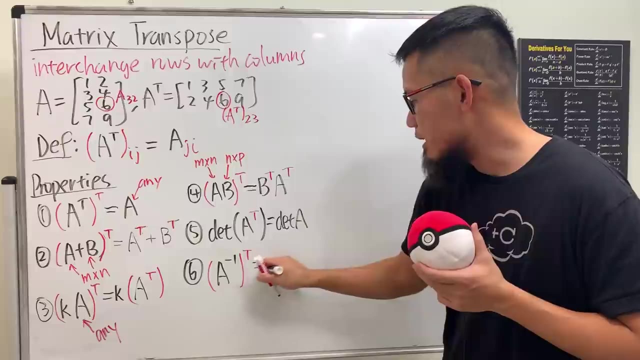 so maybe next time and perhaps the next one. number six: it's actually similar to number four. if you have a inverse- suppose you have an invertible matrix- and then you do the transpose. this right here. it's actually the same as if you do the transpose first and then look at whatever. 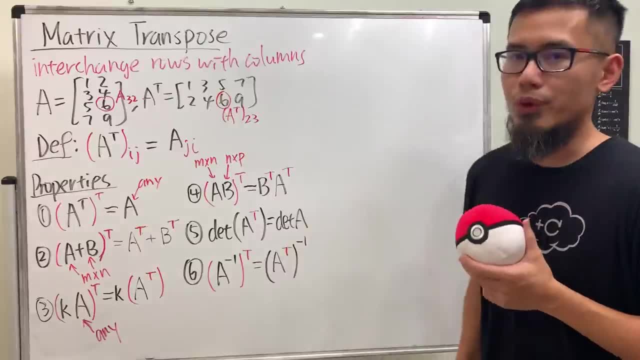 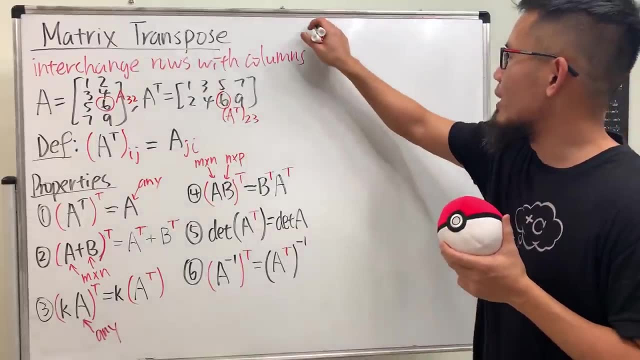 this is and do the inverse, and i think this is pretty cool. in fact, you can use this right here to help you to prove that right. so that's pretty much the ones i can come up with and i think, the common ones. if you know more, please leave a comment down below and let us know. 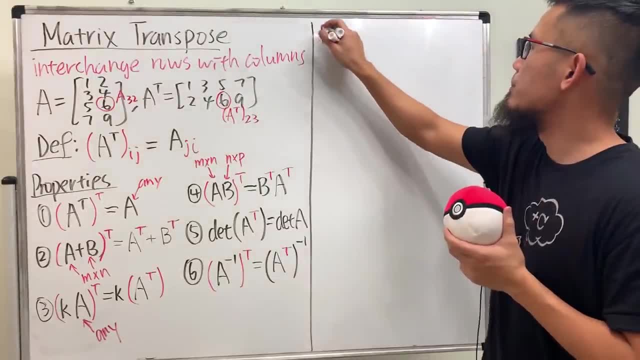 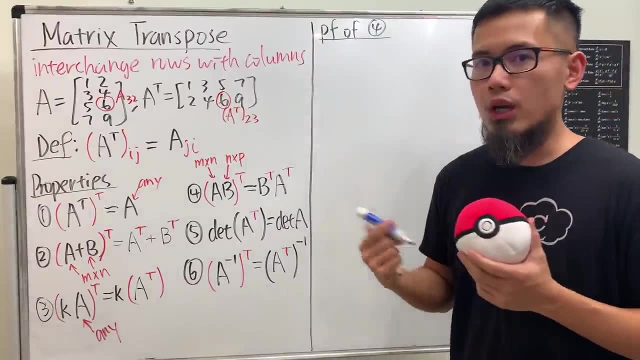 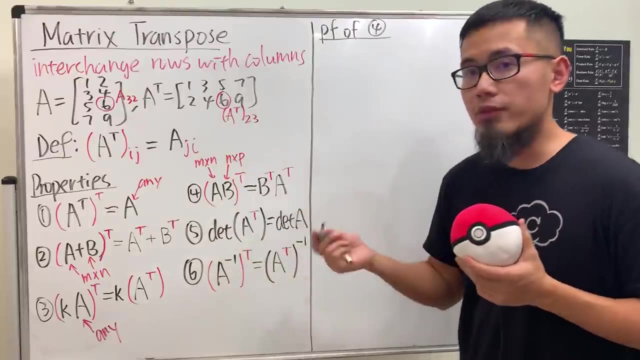 more. now, claim of five. all right, so this is just proof of property number four. and to do so, i will have to recall a few things with you guys. first, we have this right here already, but because we're talking about the product of two matrix, i will have to remember that. we have to remember that, we have to. 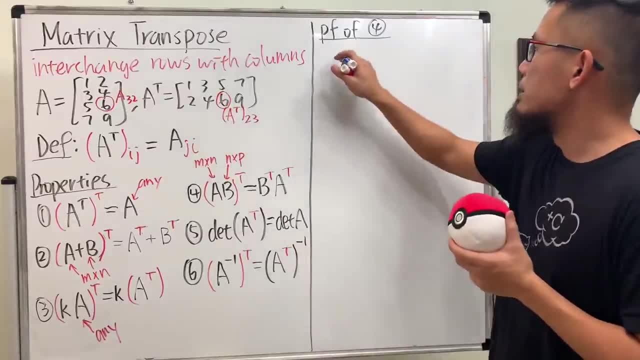 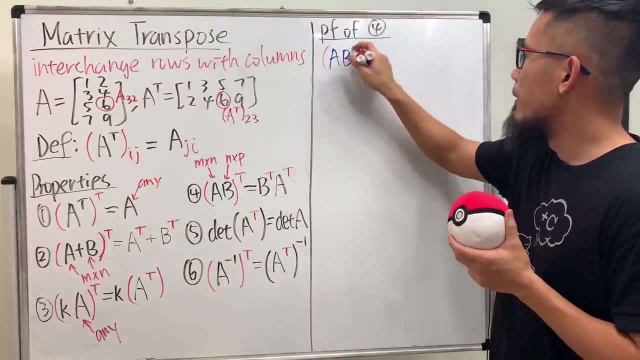 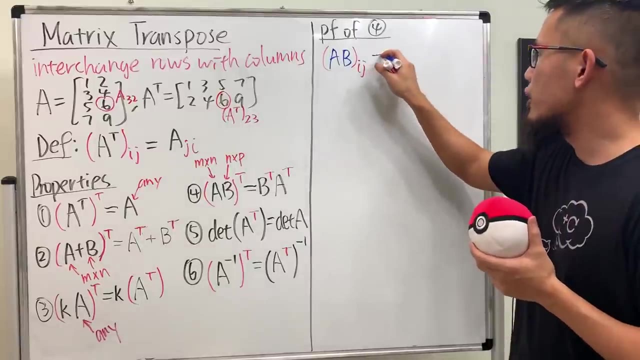 remember, guys, how we can find the product of two matrix. suppose we have a times b. of course they will have to be good dimensions. well, the key is: look at the i j entry. so let's write this down right here. this right here, you guys can check out my other video. in fact, we can write this down as: 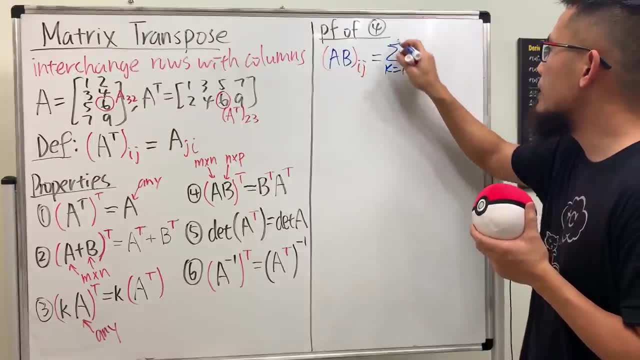 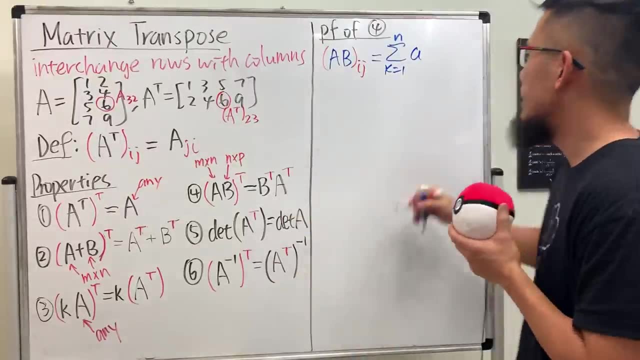 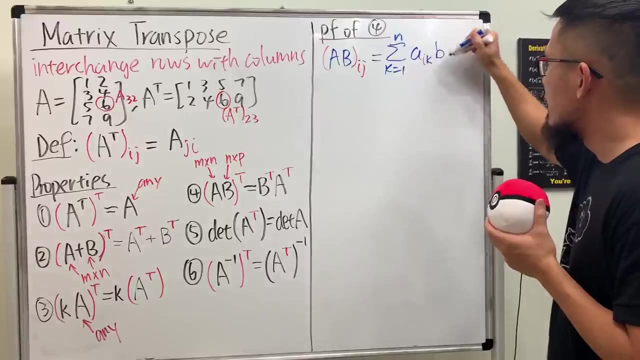 a summation. this is the sum as k goes from 1 to n and then we have little a. it's just the entry from the matrix a. but you look at the i k entry and then you multiply by b, k, j entry. so this right here is. 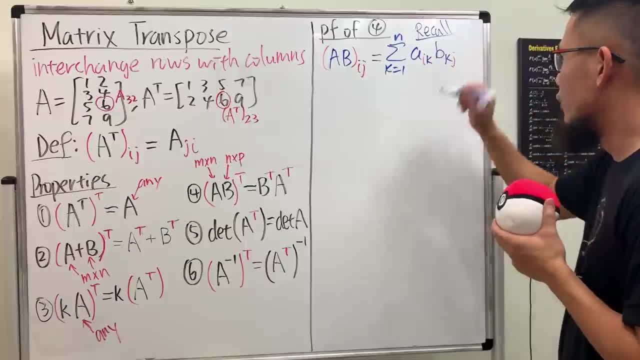 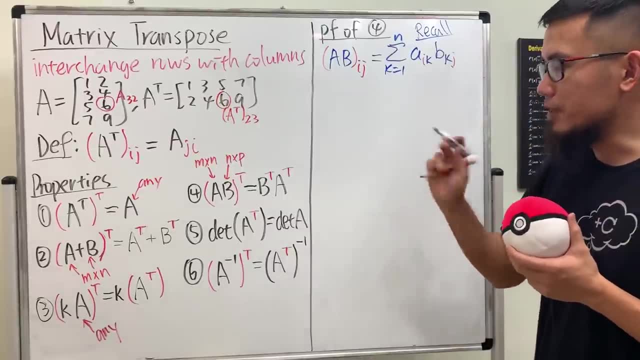 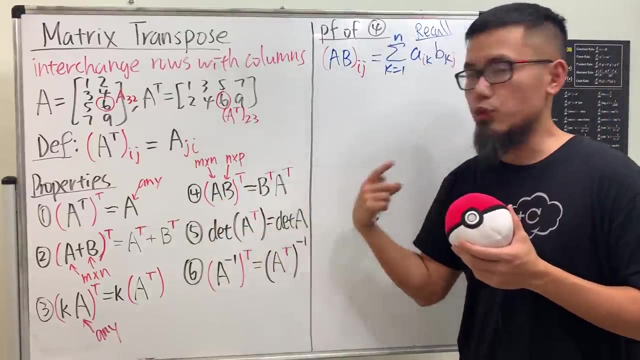 the recall and check out my other video for this product formula right here. right, so this is what we have to use to help us out. now here's the deal to prove this. we can just go from the left hand side and try to end up with the right hand side, but when we are trying to show, the transpose are equal to. 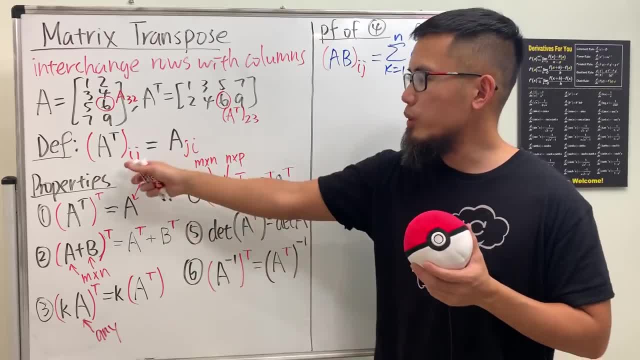 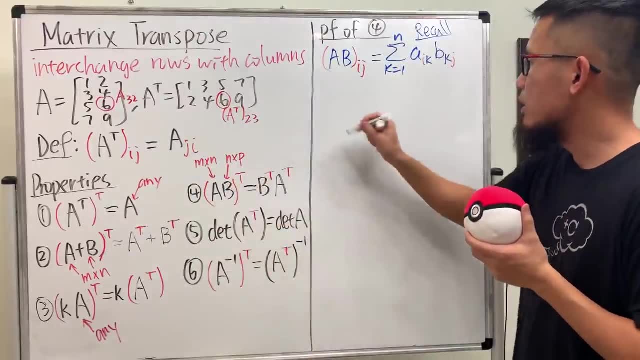 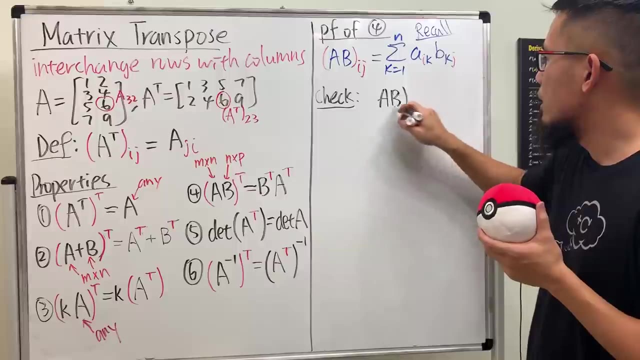 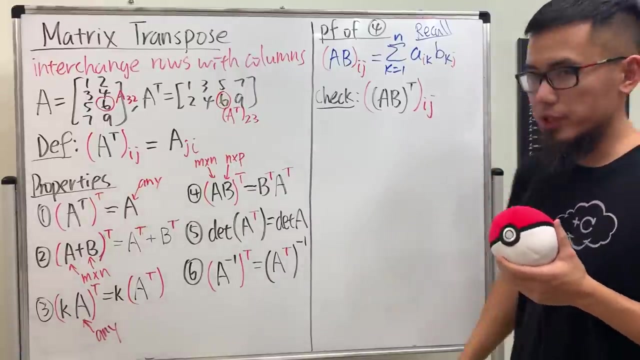 the other. all we have to do is just make sure that all the entries of the result are equal. so we'll be looking at this. so let me put this down. this is the check that we have to do. we check a, b, transpose, right, but we look at its i, j entry and hopefully we're going to be able to do this. 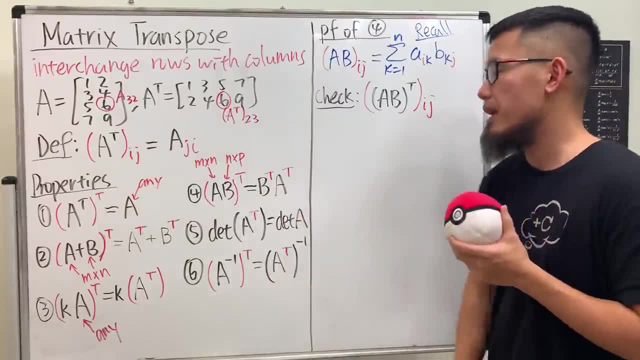 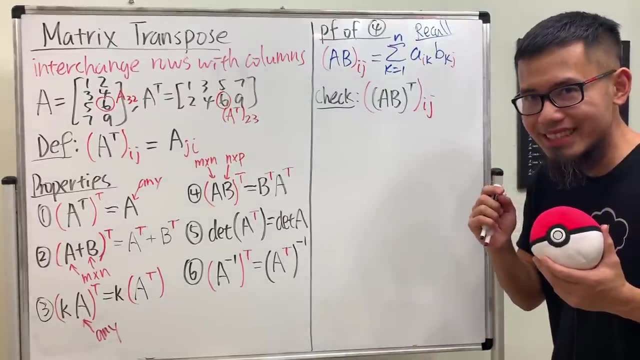 we can end up with the same i- j entry of this guy, And in that case we can say that the left-hand side and the right-hand side are equal. Now, how can we do this? First of all, to take out the transpose, all we have to do is switch the i and j. 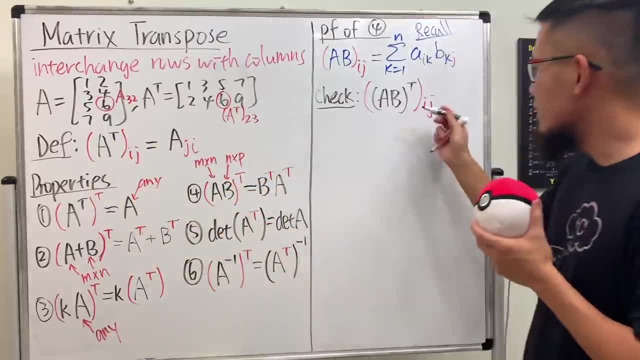 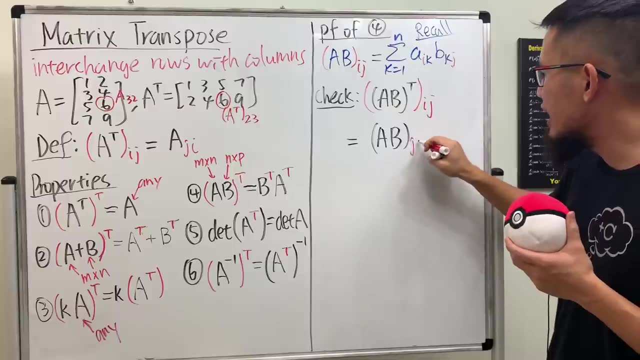 You see, to take out the transpose, we can just switch the i and j. So this right. here it's actually the same as a, b, No more transpose. but here it becomes j, i Right, So that's what we have. 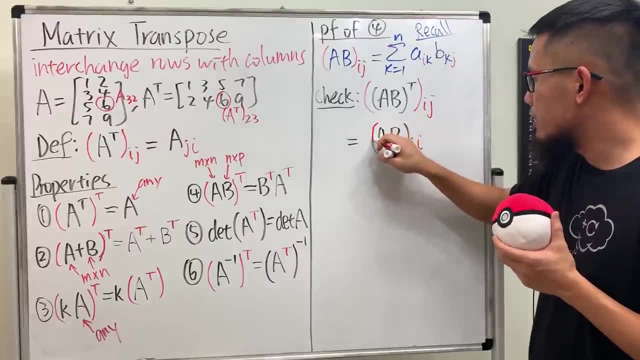 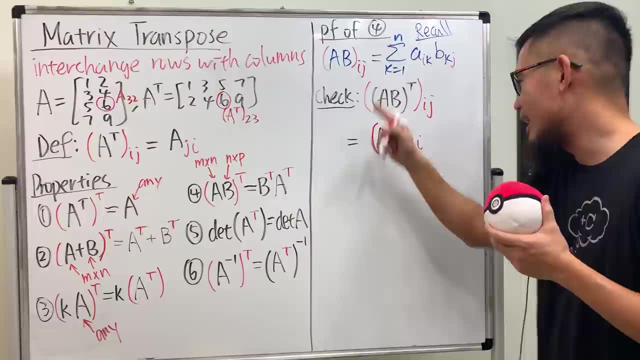 Now look at this carefully, though I'll put this down here. actually, This right here, it's almost the same as that: The red j is the blue, it's the red i. Well, anyway, the j right now is the i earlier, and then the i right now is the j earlier. 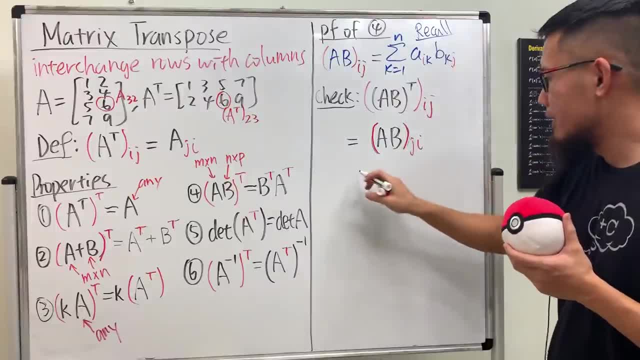 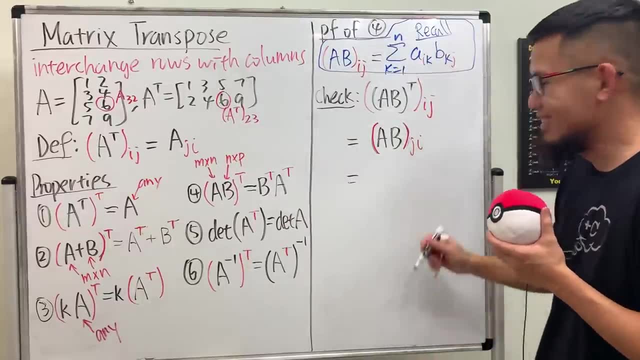 But anyway, we are going to use this umlaut right here, right? So let me just kind of box this in blue. I know, I know this is not a box, I'm sorry. Bye-bye, Here we go. 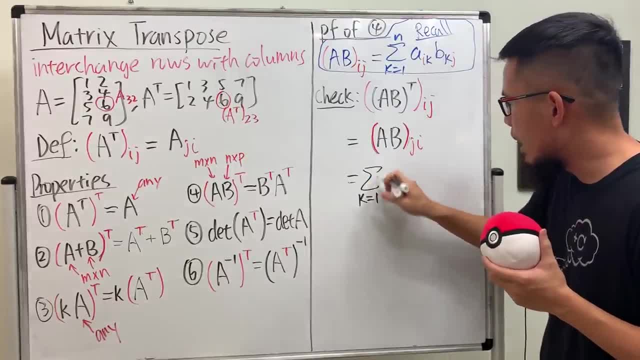 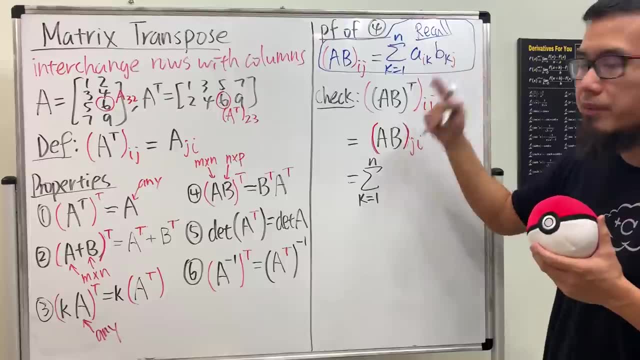 This right here it's going to be the summation. k goes from 1 to n And you see you have the i. i goes first and then, whatever this is, then just have a small letter. So here we have little a, and this time j goes first. 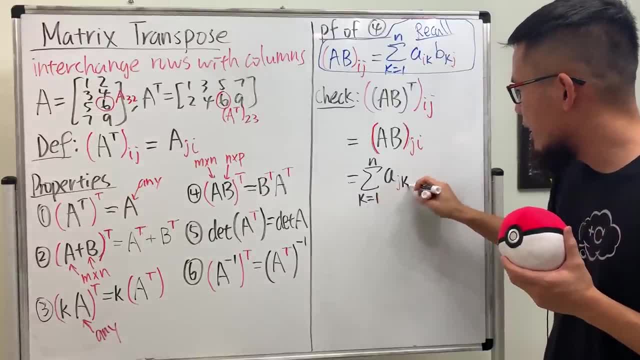 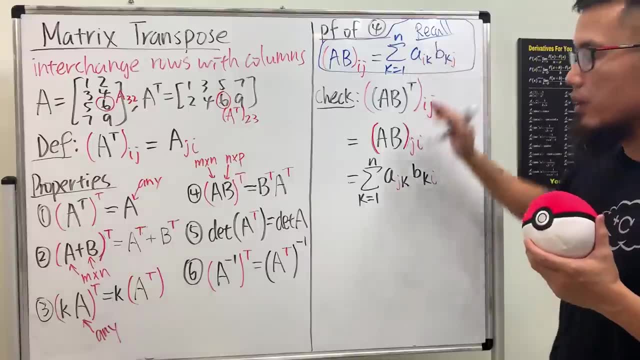 So we have j and then k and then b, and then we have the k and then we end up with i, Right? So I'm using this right here for that. It's just Because again the i and j got switched. 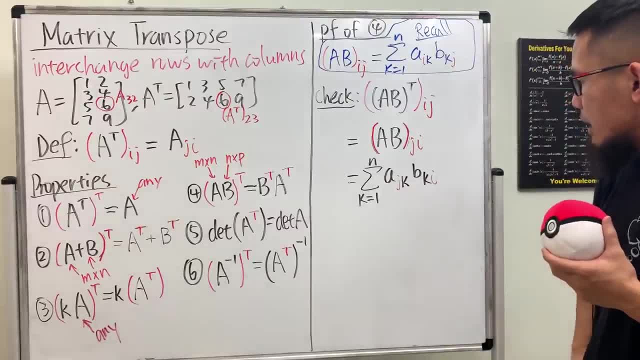 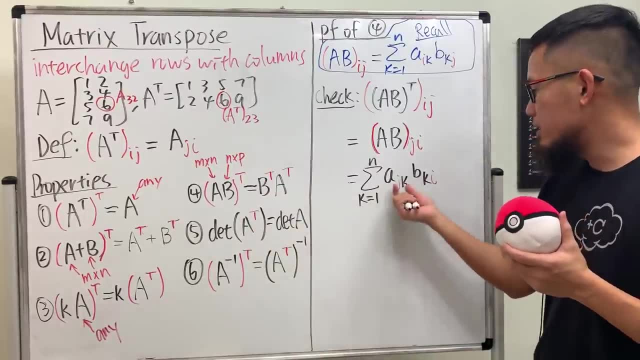 So that's what we have. Now. I kind of want to change the order right, Because that's essentially what we are trying to do right here. But we can actually just change the order right here. Why? Because this and that they are just regular numbers. 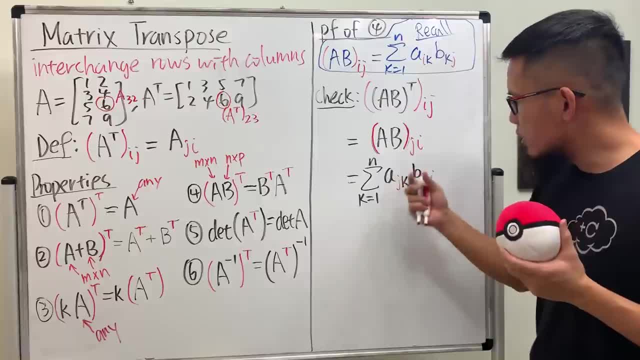 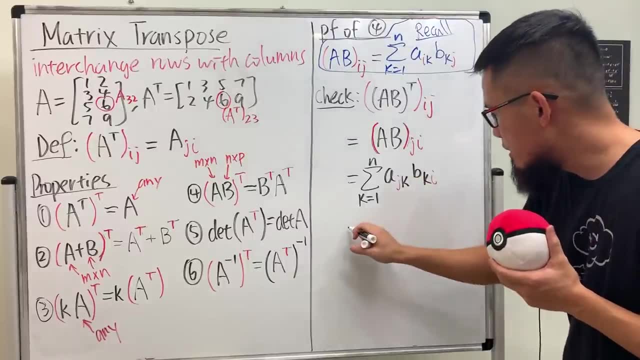 They are not matrix a, j, k is just the entry from the matrix, right? So it's just a number. So we can just reverse this. This is the same as the sum as k goes from 1 to n. 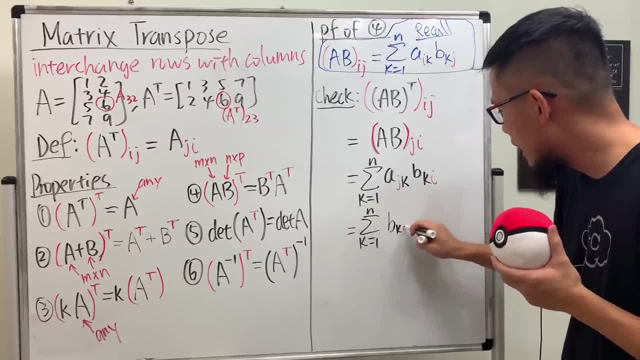 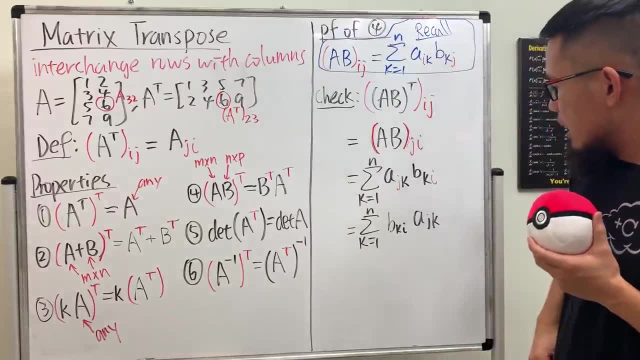 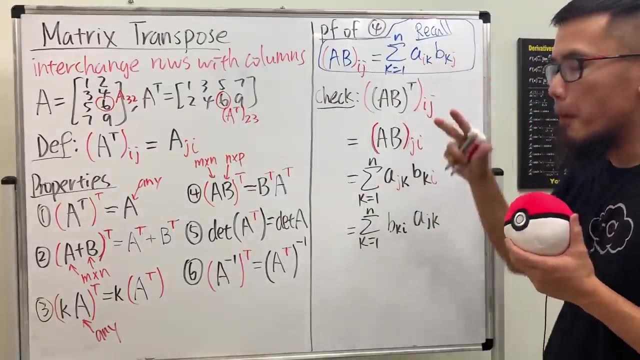 Let me put this down first. which is b k. i times a j k, That's totally the j. Now I kind of want to use this again, But if we want to do that, we will have to make sure that this and that number match. 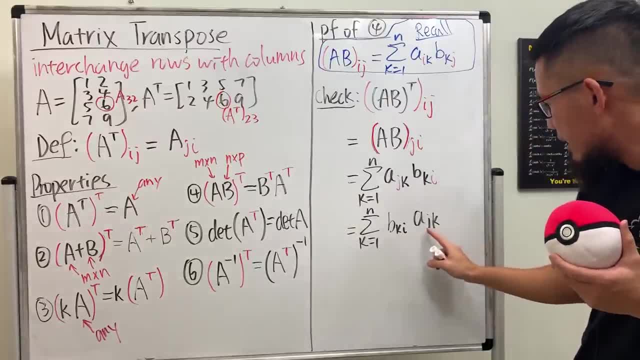 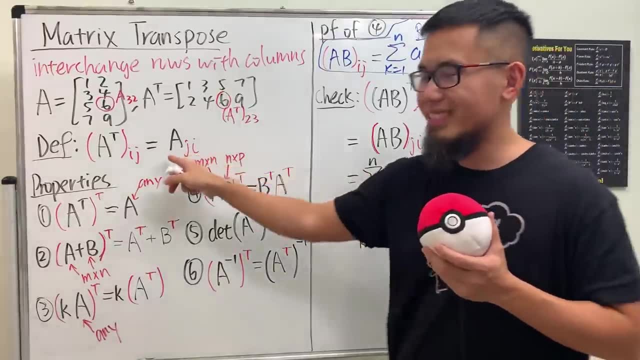 They both have to be k. I have k- i and then this is j k. I cannot reverse it, So I can reverse the index right here. We look at this, Then go back. You see we have j i. 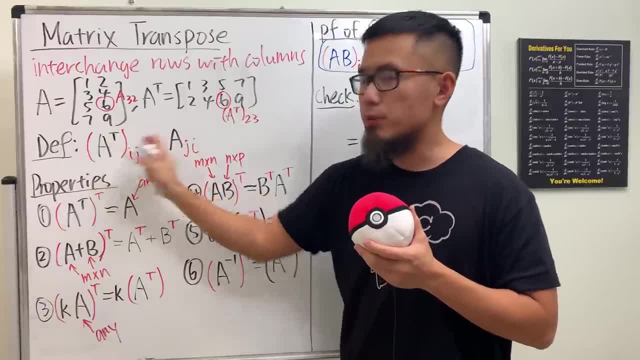 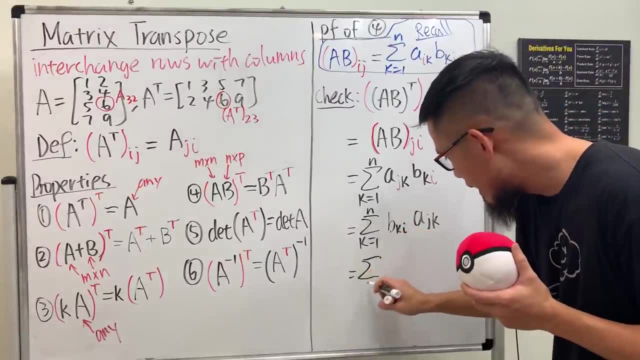 We can change that, but you just have to make sure you do the transpose right here. All right, I used little b, But right here, when I reverse, let me first write down. We have the sum as k goes from 1 to n. 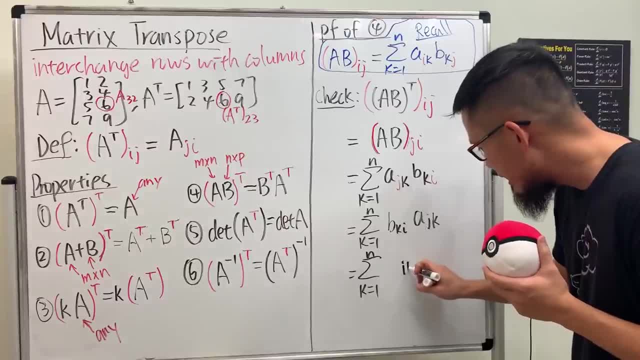 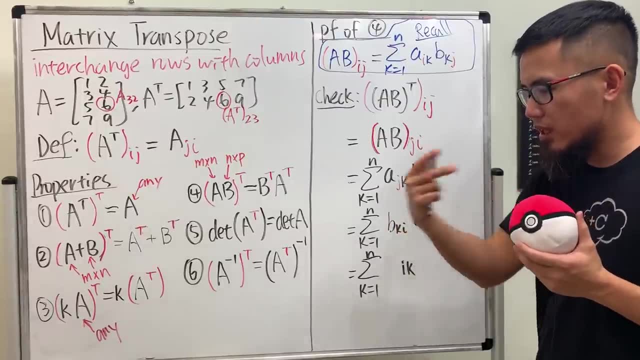 But I'm going to switch it. I want to make sure I get i k right here. But you know this. b k i is just a number from the matrix b right? Well, it's the same notation as a. 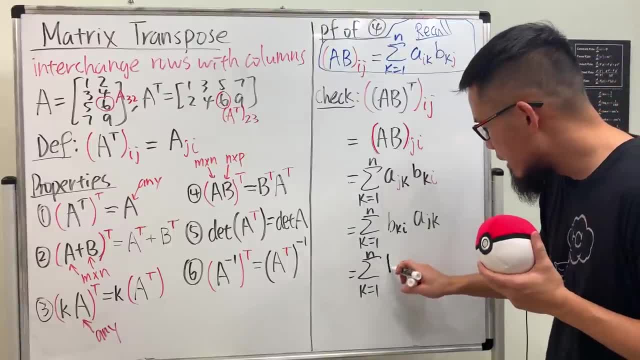 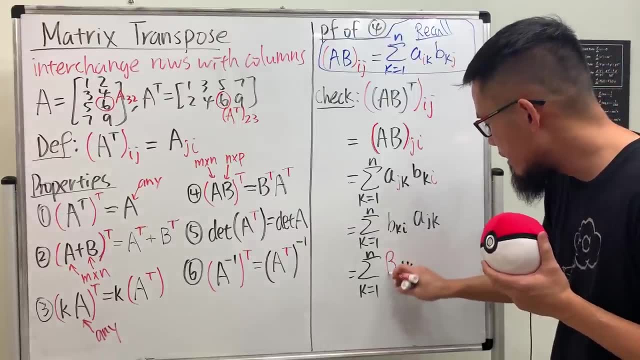 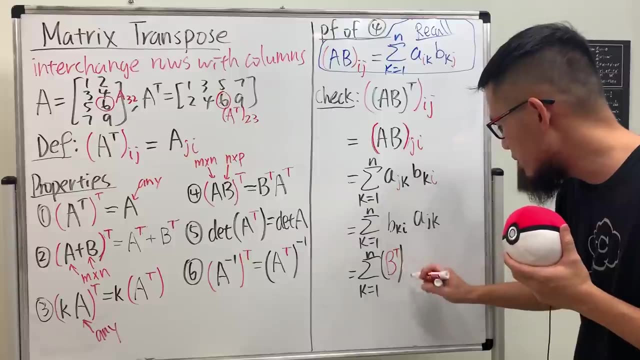 Let's look at the i case entry from the capital B right The matrix b, But we look at its transpose. So I will write down b, transpose like so. So that's the first part And again all we are doing is just using this backwards. 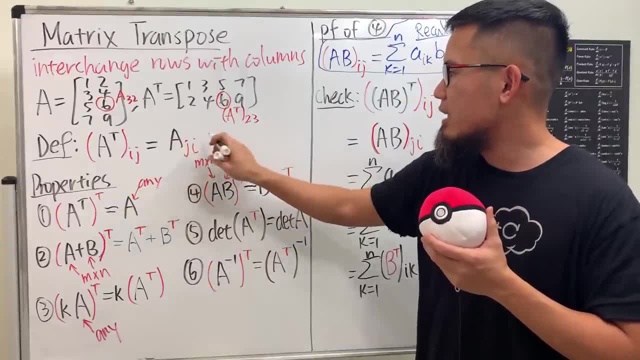 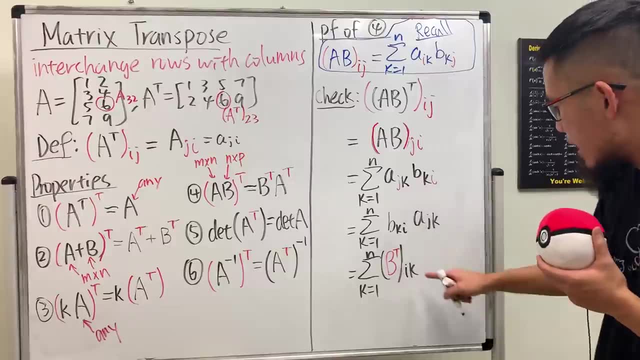 And in fact, if you have capital A j, i, this you can write here as little a j i. It's okay. Yeah, All right, Now we do the same thing. We're going to switch this and it becomes k j. 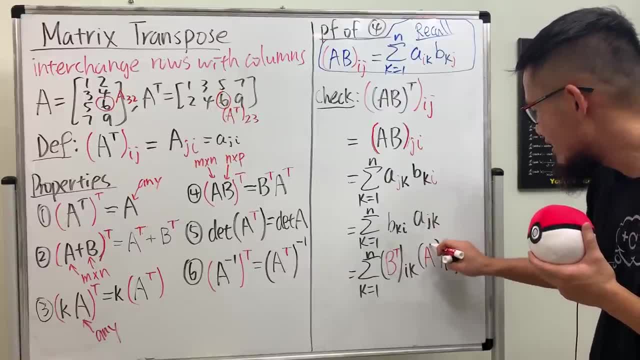 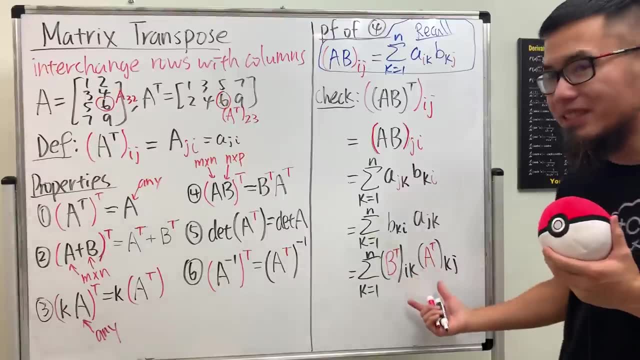 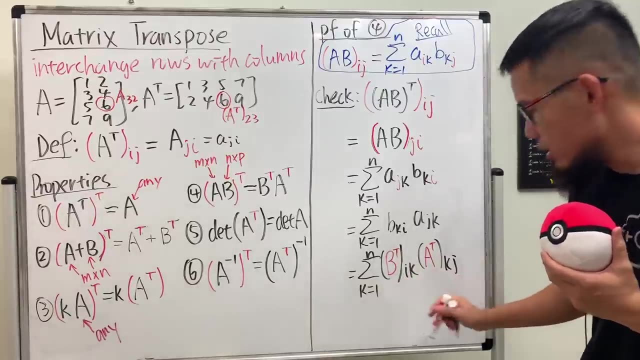 And then here I will just have a transpose. And now you see the k and k right here match right, And then we have this. So what can we do? This right here means we are looking at the i j entry right. 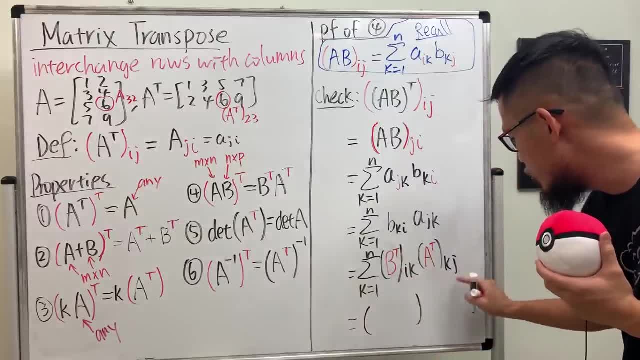 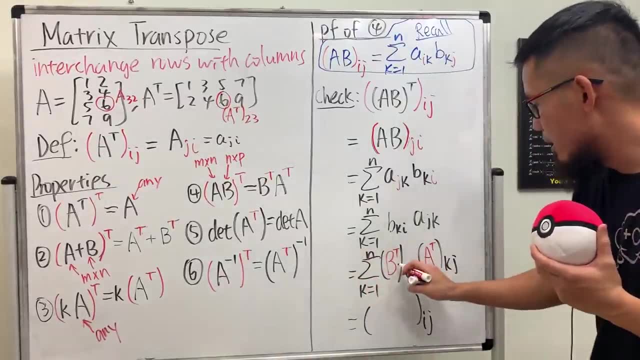 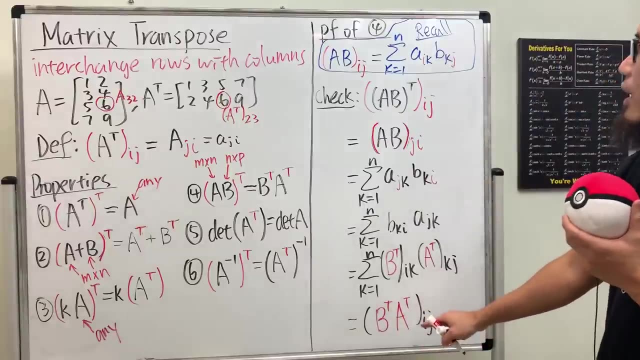 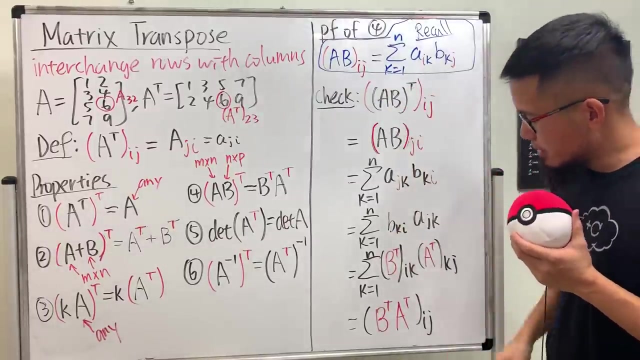 This right here means that We are looking at the i, j entry of the product of two matrices. What are they? b transpose and a transpose, And that's exactly what we have over there And, as you can see, we are saying that the entries of this thing is equal to the entry of this thing for all entries. 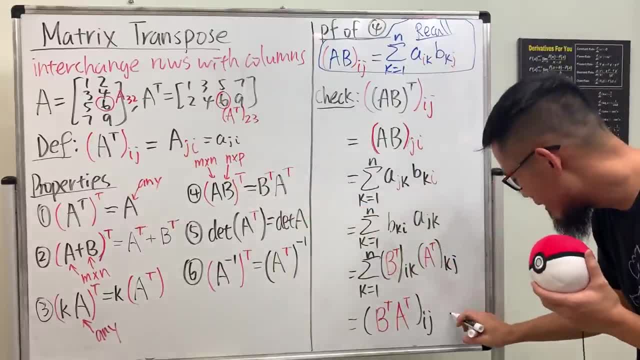 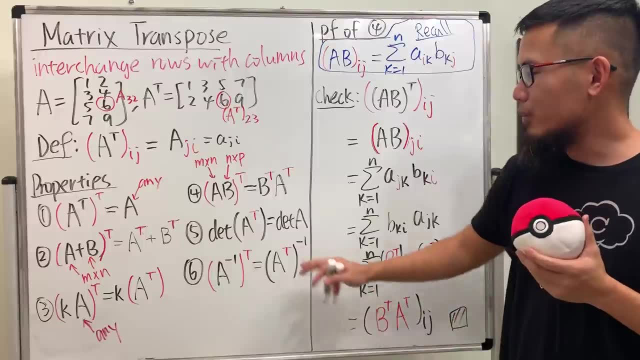 So the rest, The results, are the same. So this, right here we are done. Very nice. Right Now you guys can think about how to prove five and six, And the hint to prove six is you can use number four. 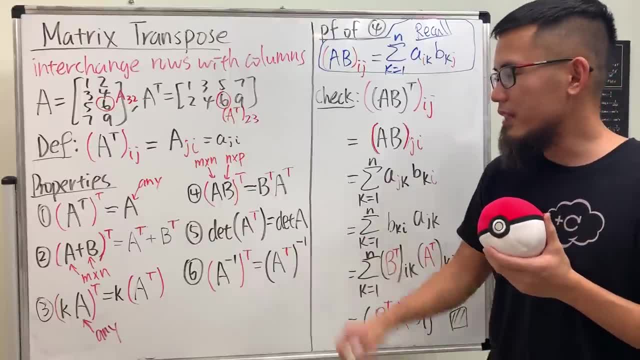 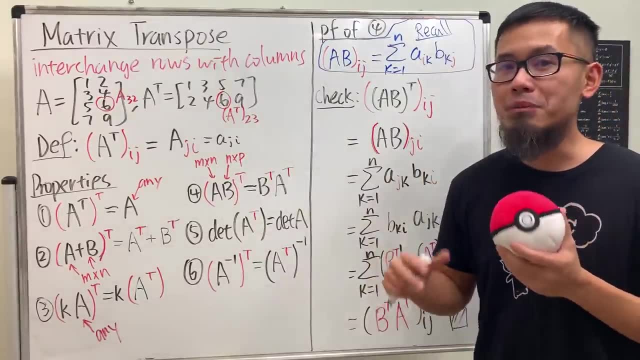 And for this maybe use the cofactor or other method, And then, if you have any other properties, leave a comment down below and let me know. At the moment, that's it Coming up. next I will do some symmetric matrix for you guys with some little proof. 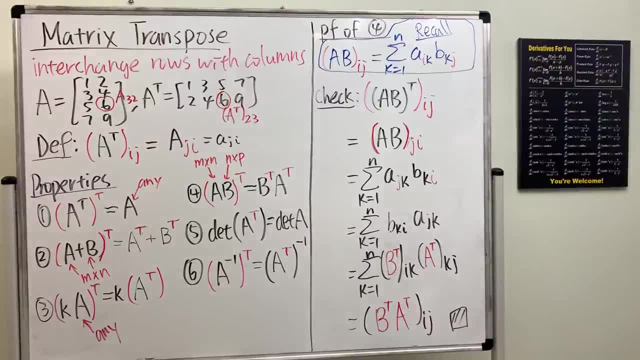 Right, That's it, Thank you.